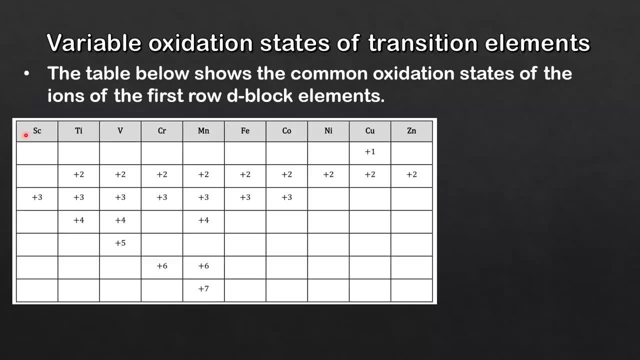 first row d-block elements. The first row d-block elements include the elements from scandium to zinc. However, zinc is not considered a transition element, so from now on I'm going to blank out the zinc column So, as you can see, all the transition elements except scandium. 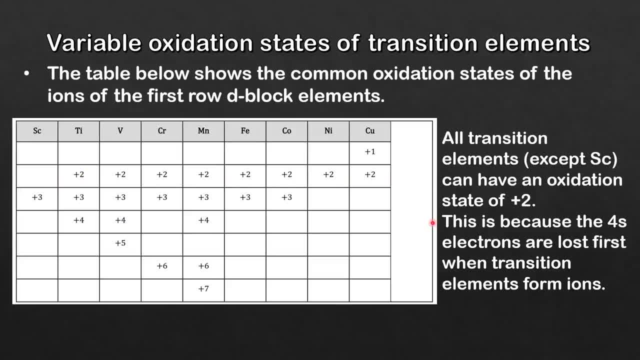 can have an oxidation state of plus 2.. This is because the 4s electrons are lost first when transition elements form ions: The majority of the transition metals, such as titanium, vanadium, chromium, manganese, iron, cobalt and copper. they have variable oxidation states, with manganese having 5 and the highest. 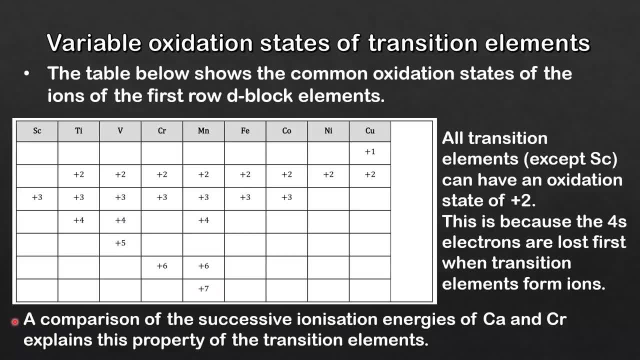 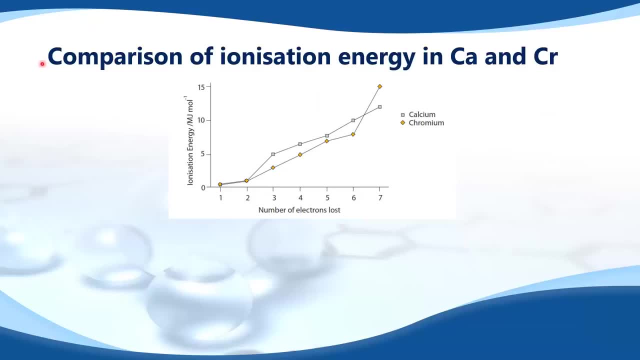 being plus 7.. A comparison of the successive ionization energies of calcium, which is an s-block element, and chromium, which is a transition element, explains this property of the transition elements, and that's what we'll look at next, So to understand why transition metals have. 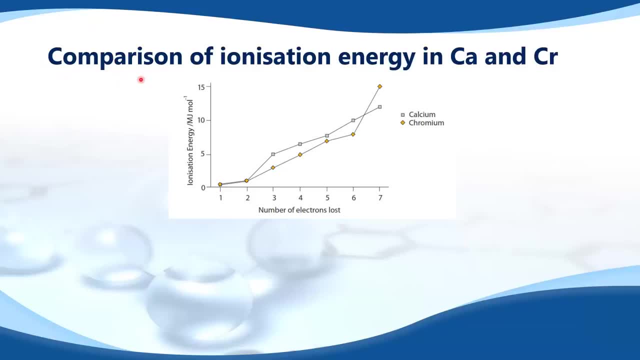 variable oxidation states. we'll have a look at the comparison of successive ionization energies in calcium and chromium. So if we look at calcium first, you see a big increase between the second and third ionization energy. So we look at the electron configuration for calcium, the 4s electrons are lost first and then this: 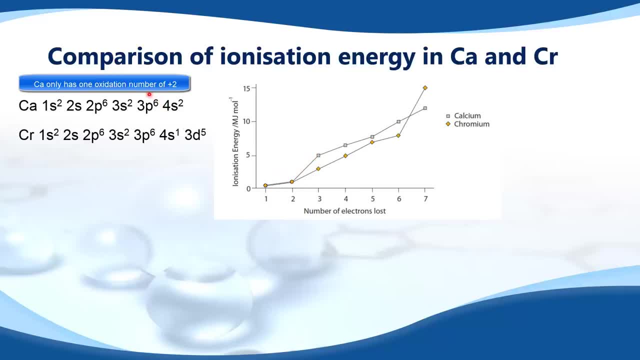 big jump in ionization energy corresponds to the electron being removed from the 3p sublevel is at a lower energy than the 4s. It's also closer to the nucleus so there's a stronger electrostatic attraction holding the electrons. so more energy is required to remove the third. 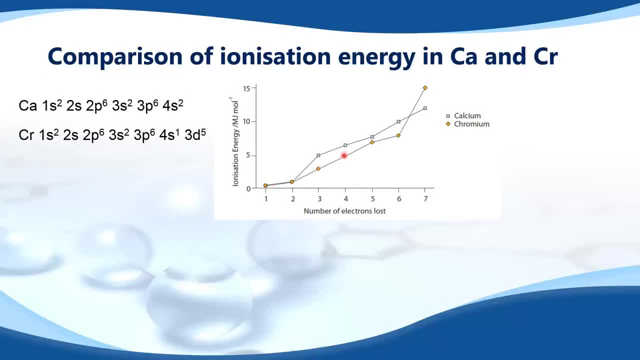 electron. So if we look at the successive ionization energies for chromium, we don't see the big jump until the seventh electron is being removed. And the reason for this big jump is the seventh electron is being removed from the 3p sublevel. The first six electrons that are 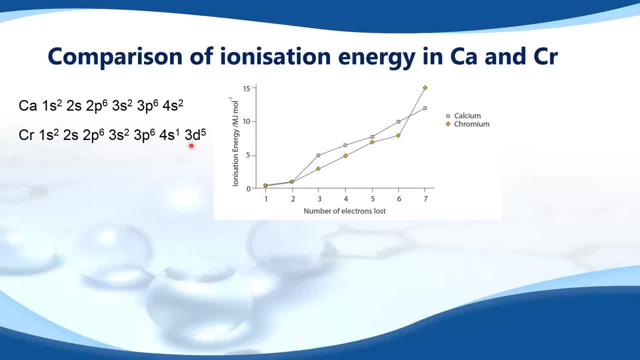 removed. they are being taken from the 4s and 3d sublevels. Because the 4s and 3d sublevels are quite close in energy, there's no big jump until we remove the electron from the 3p sublevel.